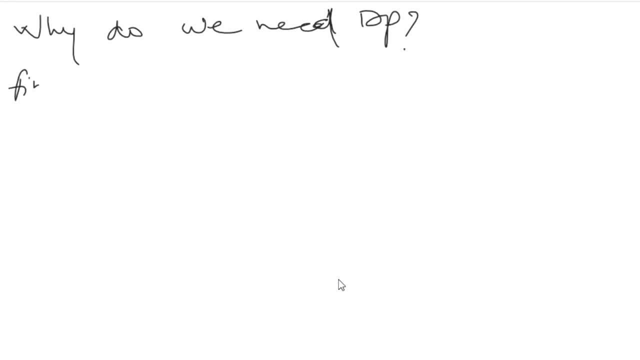 last two terms. so fib of n is fib of n minus 1 plus fib of n minus 2.. now if we try to implement this relation directly using divide and conquer technique, then there will be use problems. let's see what. so you will see that fib of n is sum of fib of n minus 1. 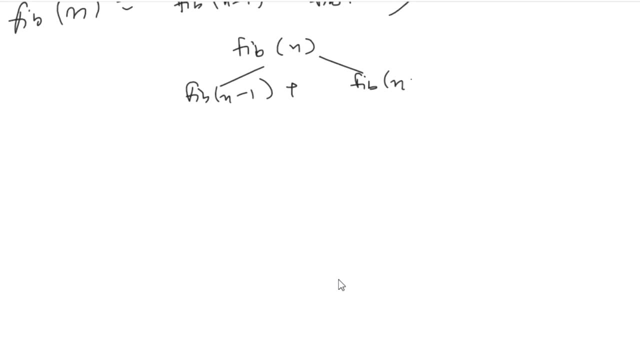 and fib of n minus 2, and again, fib of n minus 1 is sum of fib of n minus 1 plus n minus 2, plus n minus 3, and for fib of n minus 2 it will be n minus 3 and n minus 4.. so, as you can see that, 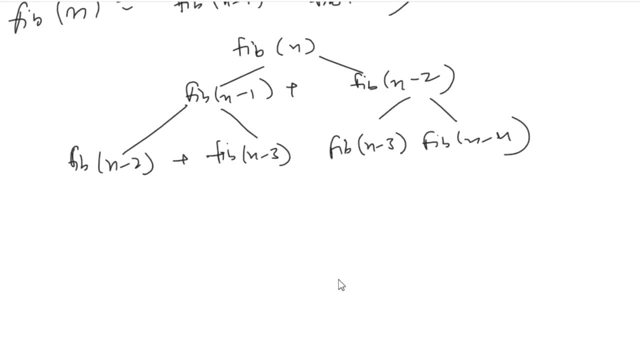 this tree will unfold in n steps, i mean until n will become 1, so n n minus 1, n minus 2 until fib of 1. so there will. the height of the tree will be n and in each step the number of sub problems are: 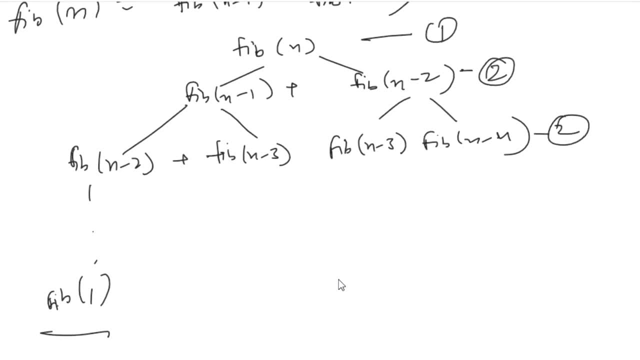 multiplied by 2, they are increasing by the factor of 2, so ultimately there will be 2 to the power n sub problems. so to solve just a problem of size n, we have to solve total 2 to the power n sub problems, and this is pretty bad. so the time complexity of our algorithm is o of. 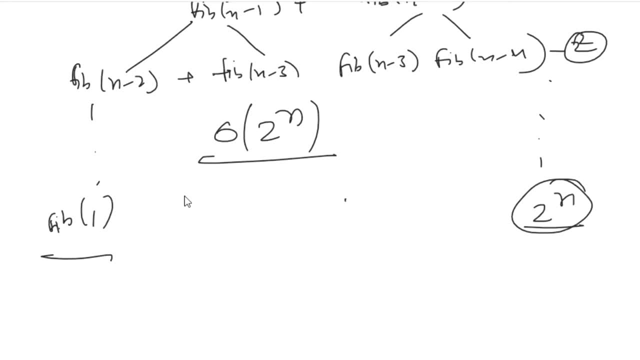 2 to the power n. this is not good so we need to do something on that. so let me add up page before moving forward and let me rename it. rename page and page two: okay, so let's see how many sub problems fib of n can have. 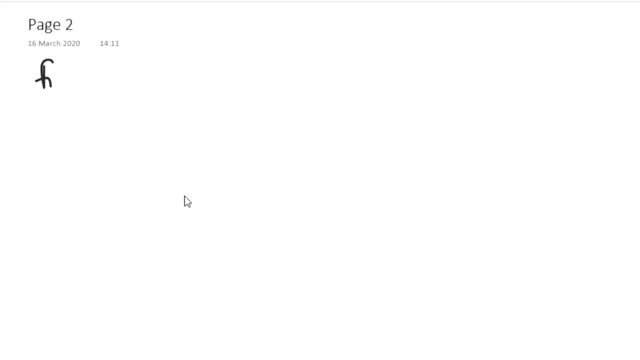 fib of n can have five problems can have. so fave of n is we need fave of n minus 1 and fave of n minus 2. now for them we need fave of n minus 3. for fave of n minus 3 we need fave of n minus 4 and fave of n minus. 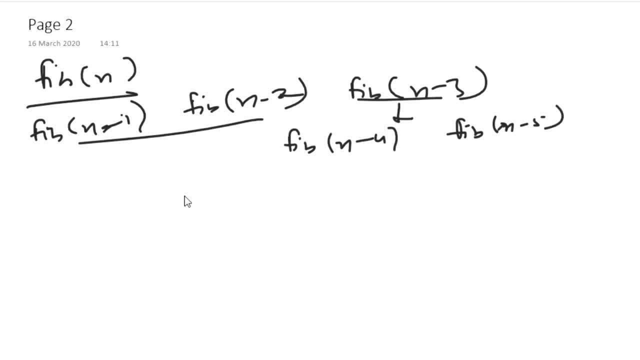 5. so in total, at most we will go till fave of 1 and there will be only n minus 1 sub problems and still we are completing total of 2 to the power n sub problems, which means we are doing something wrong. so let's see what we are doing wrong. so fave of 5 if you. 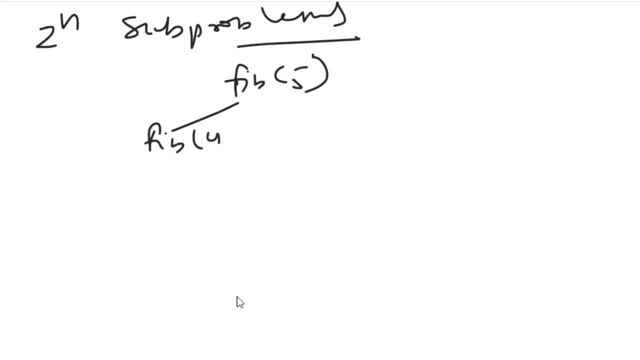 try to see that fave of 5 is fave of 4 and fave of 3 and further, fave of 4 is fave of 3 and fave of 2, so you can see that we are completing fave of 3 two times. 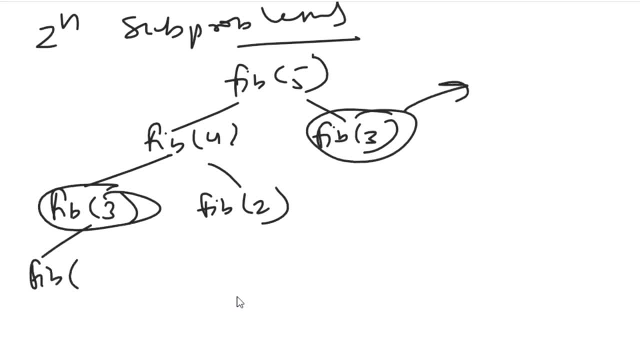 and if you further unfold this tree, then you will see that we are computing fave of 2, three times. so all these multiple solving of sub problems is leading to this exponential number of sub problems. so what you are seeing is this is called overlapping of sub problems. 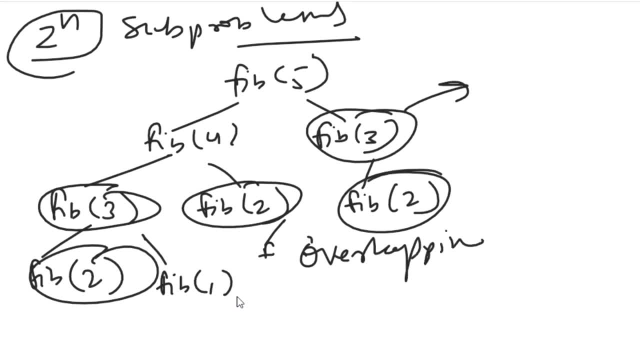 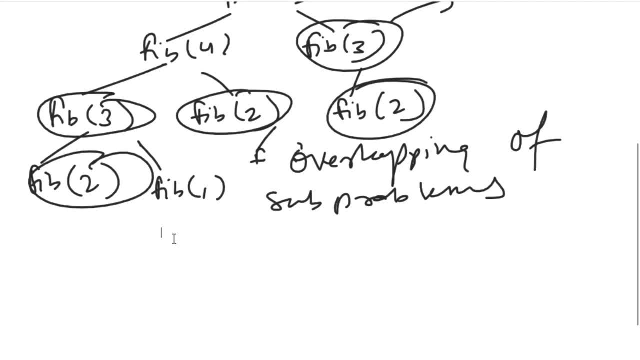 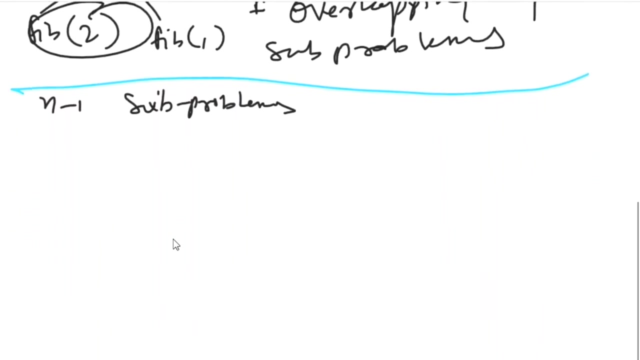 overlapping of problems and we need to stop this, to improve our algorithm, to optimize our algorithm. so let's see how we can do that. so there are total of n minus 1 sub problems, sub problems, and then there is one more nth problem. in total, we have n problems to solve. 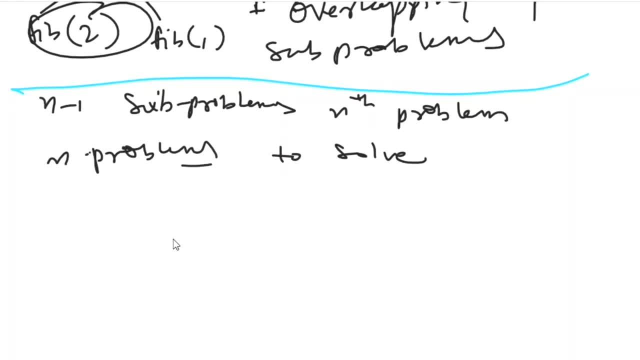 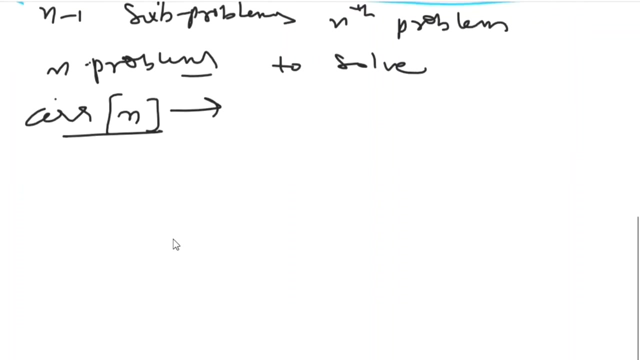 to solve. so instead of recomputing them, what we can do is we can compute them once and store them in a in an array of size m. so this will allow us to reuse the solutions of the sub problems. let's see how we can do that. so if fib of n is if we have computed, let's say if already. 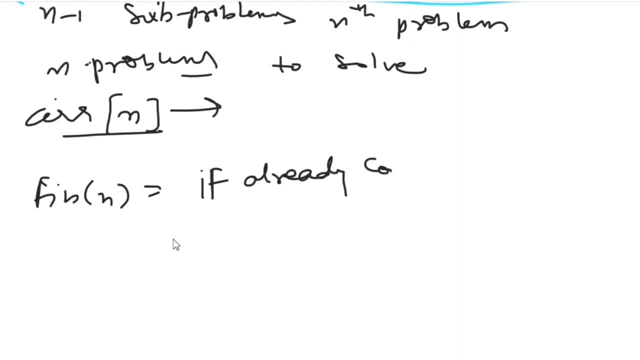 computed, then just return array of n, then, if not computed, then compute and finally assign array n to computed value and then return fib of return array of n. so let's see how we can apply it for a general recursion. so you have a function f and there are some arguments. 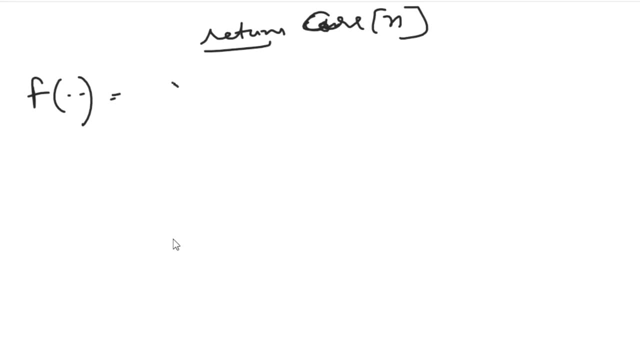 in it. okay, there will be. so its structure is base case, form something- and then return value so we can modify this recursion like this. so do like this: f is base case. now add a check of already computed. if already computed, then use, return it from r array, and if not computed, then compute it and when you obtain, 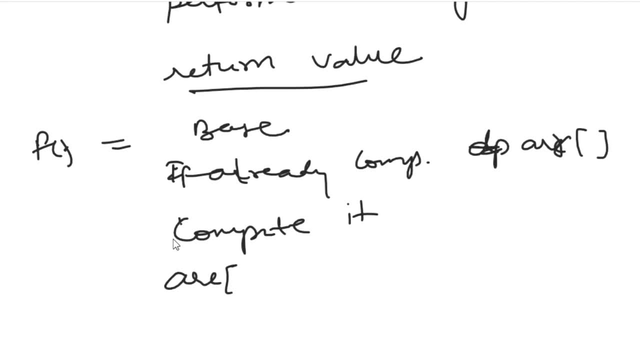 a value, assign it to array means the corresponding index at corresponding index, okay, and then finally return value. so this is the way of extending a recursion to recursive solution, to a dynamic programming solution. so i'll show you an example of a problem. it's a, it's a, it's a standard problem. 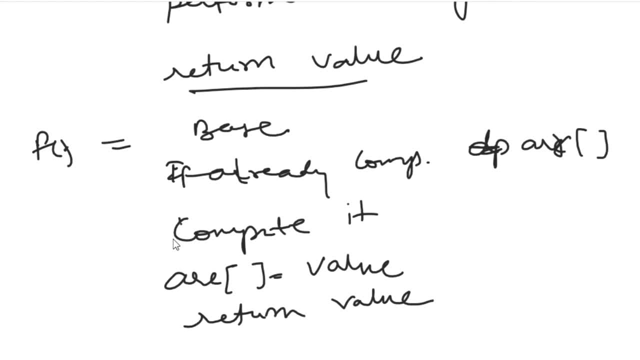 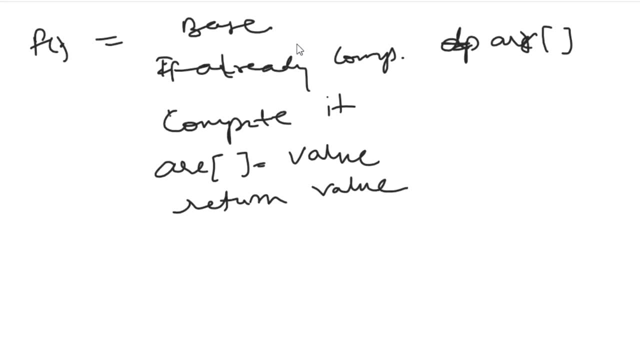 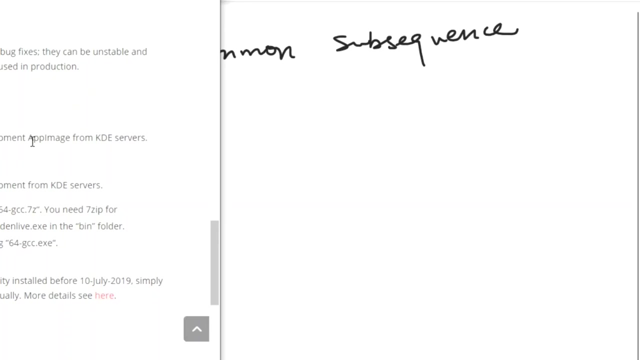 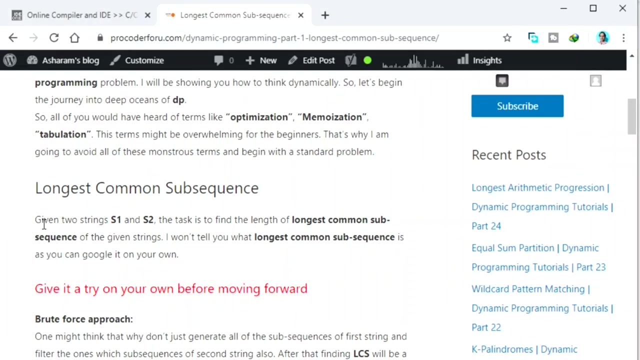 you all would avoid of it longest common subsequence. so now let's see how to solve longest common subsequence problem using recursional dynamic programming. so page 3: okay, now longest common subsequence. so let's see the problem statement. first wait, wait, sorry, okay, okay. so given two strings, s1 and s2. okay, we are given two strings, s1 and s2. 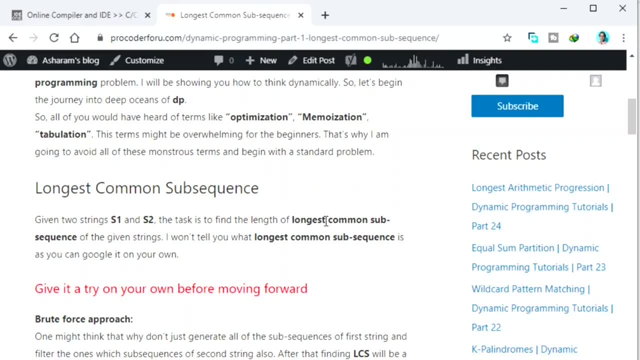 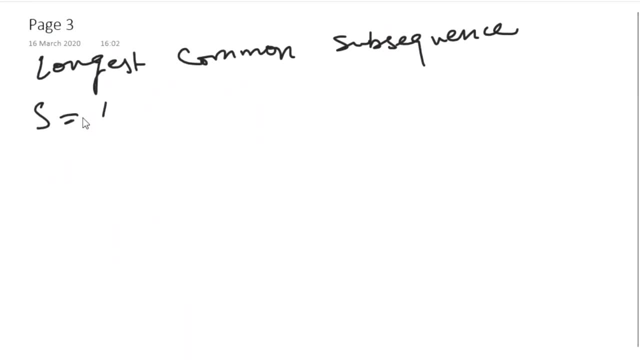 and your task is to find the length of longest common subsequence. so, first of all, what is it? what is the subsequence? so let's say you have given a string, s equal to a, b, c, d, e. now you delete certain characters, any number of characters like 0, 1, 2, 3 or 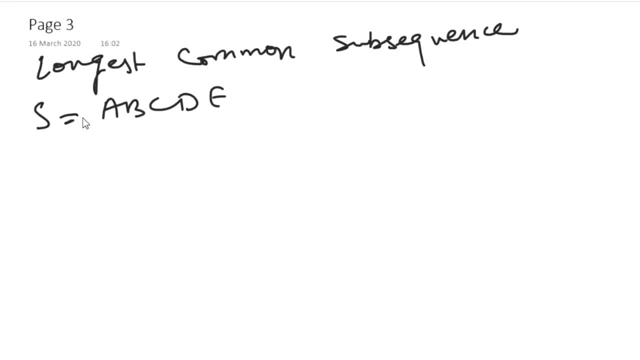 delete the whole string, so whatever left will be the subsequence of that string. suppose you delete a and e, so the subsequence will be a, c, e. suppose you delete b, c, d, then it will be a- e. suppose you delete whole a, b, c, d, e, then subsequence will be empty string. so now our task is: 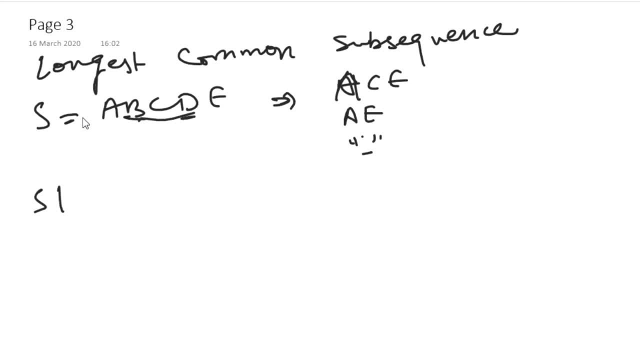 let. you are given with two string, s1 and s1. let's say s1 is a, b, c, d, e, f, and your s2 is: let's say c, d, f, d, e, g, e. don't include the g. okay, let say th. no wait, let's say okay, this fine, so length. 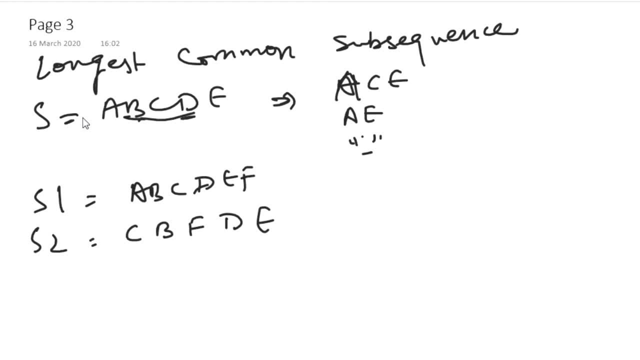 of s1 and s2 can vary means they can differ, ok, or they can be equal, so longest common subsequence for this pair, s1 and s2, is. so let's say you have given on your first string s1 and s 2 are equal characters. this means on your first string is equal, correctly so. 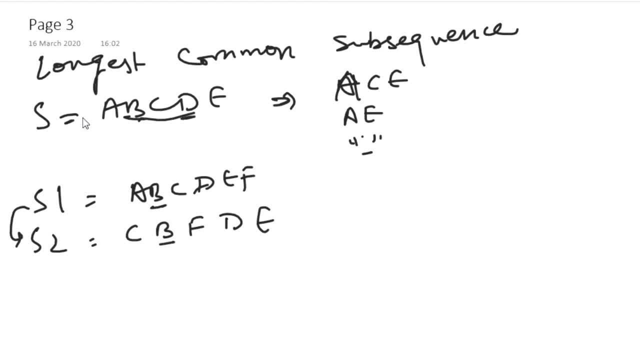 have B here, B here, and then you have D here and then E here. okay, so so it will be B, D, E, longer longest common subsequence. so length of longest common subsequence is LLCS is 3. so now we have to write an algorithm for. 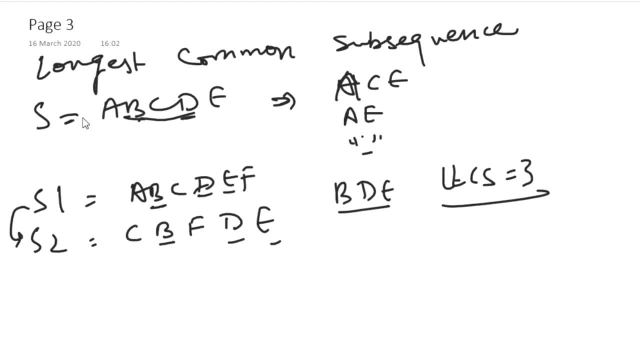 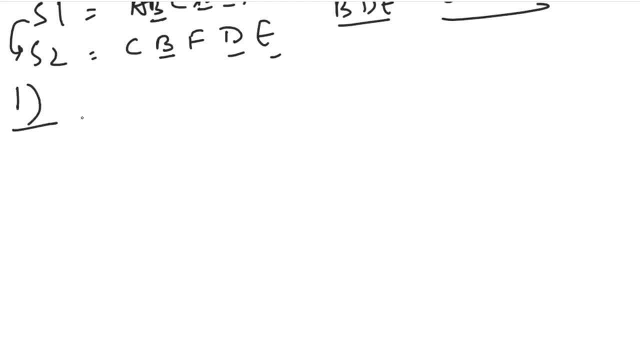 general, two general strings: S1 and S2. let's see how to do that, sir. first step is to find a recursive brute force solution. remember that you have to find a recursive solution. remember that you have to find a recursive solution. remember that you have to find a recursive solution, not an iterative one, because you can easily. 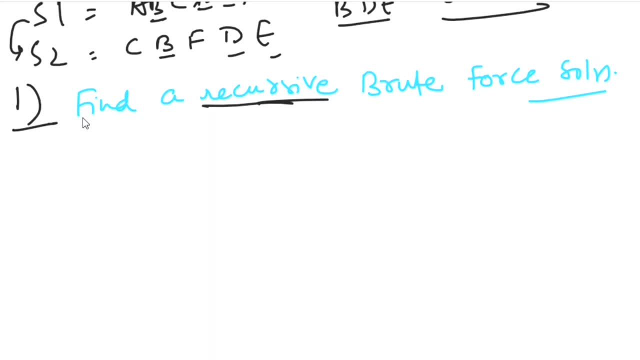 optimize a recursive solution, but it can be sometimes difficult to optimize the iterative one also. usually when the number of subproblems are like 2 to the par n, then iterative solutions are not. that means implementation of iterative solutions is not easy. okay, so find a recursive brute force solution. 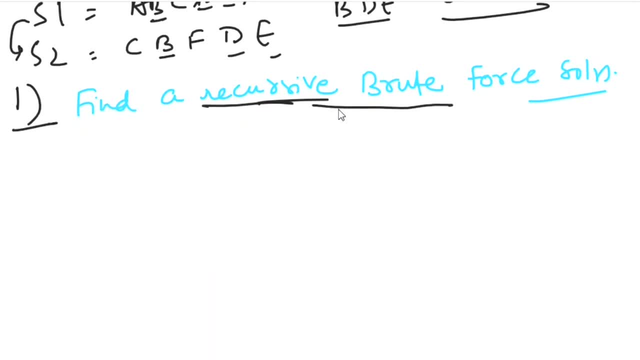 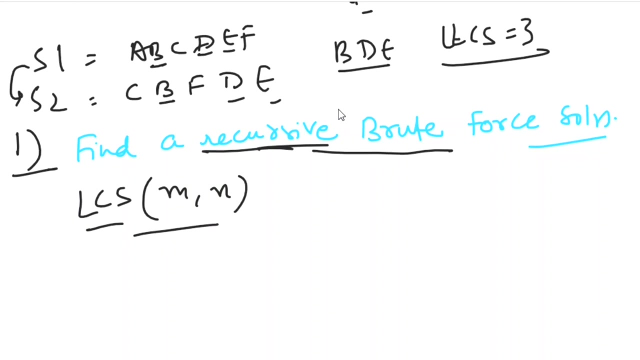 okay, so let's see what we can do for this to. let's consider this. let's consider functional LCS with length m and n, so we'll analyze means we'll you have to analyze S1 and S2, so you need a reference for that. so we are taking the last characters of S1 and S2 as reference. 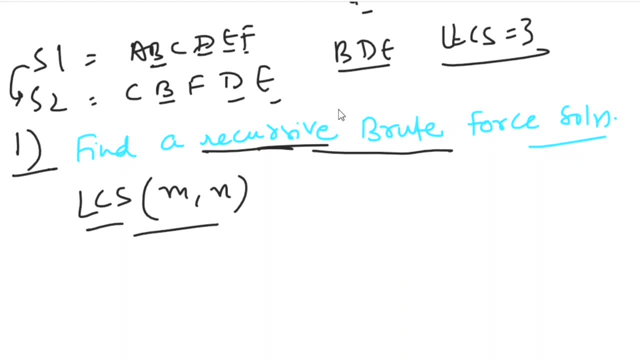 so if these characters are equal, last characters are equal, though they are not in this pair. but let's say we have a pair: a, b, c and c, d, c. let's say e, d, c. so if they are equal, last characters are equal, then this character c, that last character, will definitely be a part of 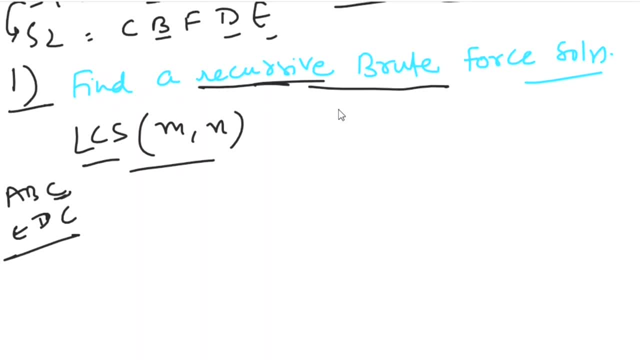 our longest common subsequence. because let's say, if you don't include that character in your longest common subsequence, then you exclude this, then there is no c in that, so our longest common subsequence will be empty string. so it's a greedy use. you can say it's a greedy. 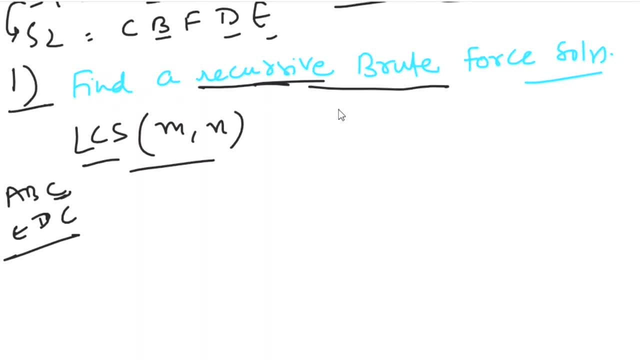 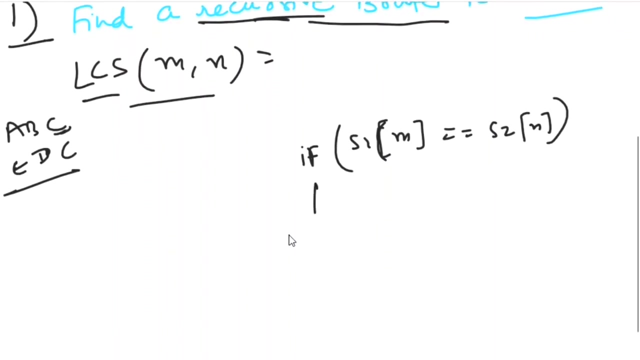 statement that you have to include them last characters if they are equal. so if the last characters are equal, if s1, s1 of m equals to so s2 of n, then our problem will reduce to means, our length will increase by one and our problem will reduce to m minus 1 comma, n minus 1, because we can't reuse the last characters. 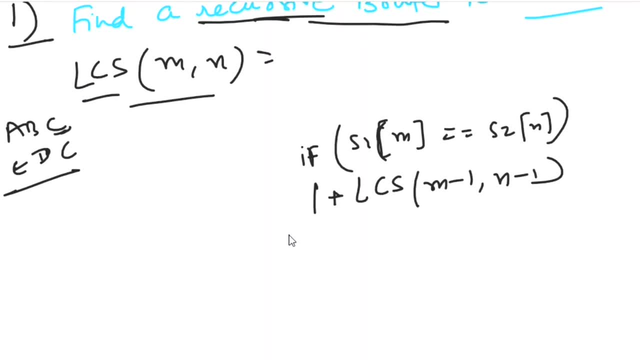 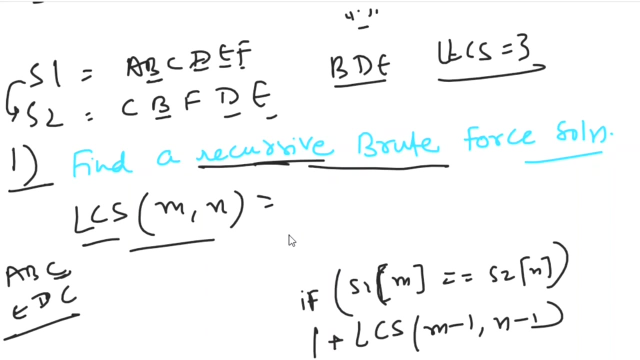 once we have included it in our longest common subsequence. now there will be another case when they are not equal. in that case, what we can do is: we don't use it means, so exclude it from our solution and we compare the remaining s2 and the s1. or we can do is: 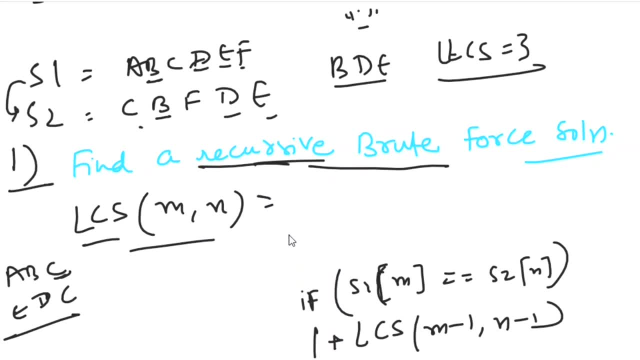 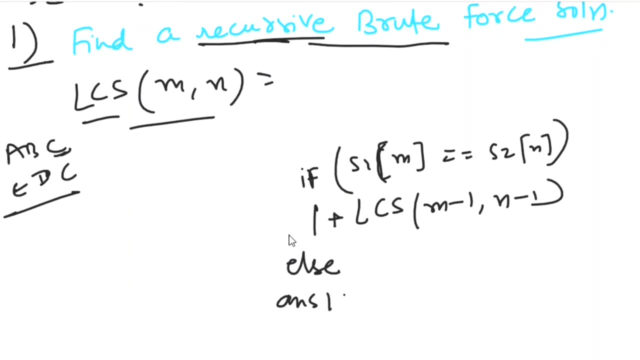 exclude last character of s1 and compare s1 and s2, remaining s1 and s2. so okay. so let's see what we can do. so our answer one is: exclude the first, correct last character of s1, so lcs m minus 1 comma n. remember that. uh, it is not contributing to the length of longest. 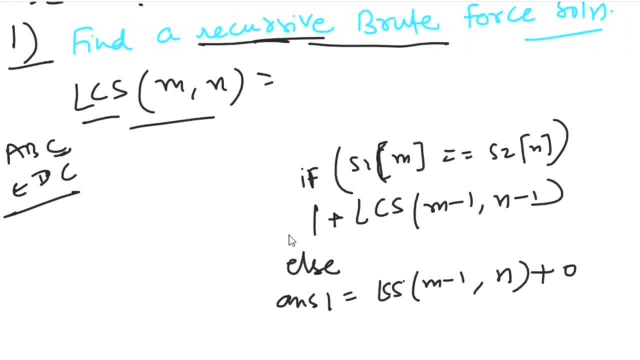 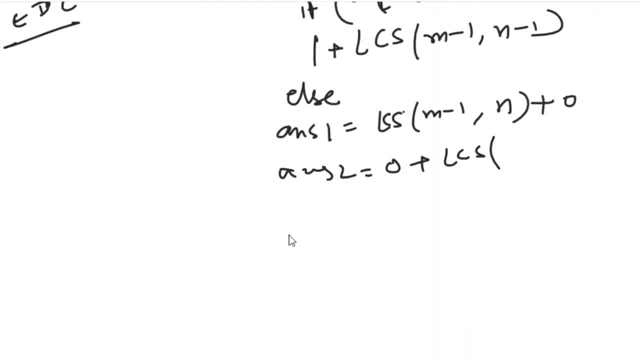 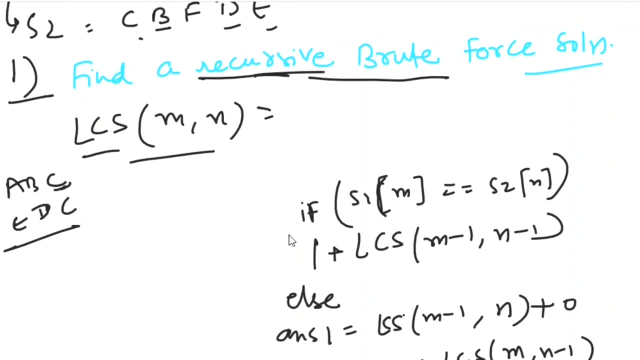 commercial sequence. therefore we are adding 0 to it and answer 2 is 0 plus lcs m comma n minus 1. so this is our recursive solution. only thing is left is to find base cases for it. so if either m is 0 or either n is 0, that 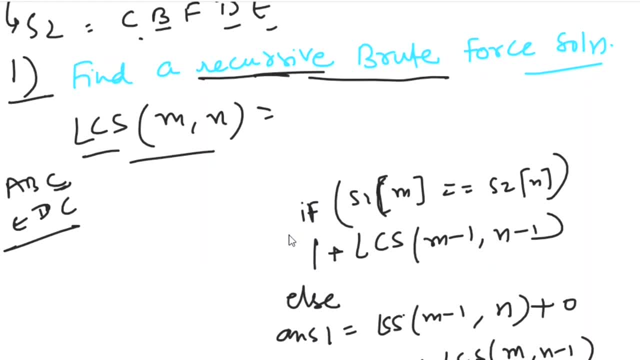 is. that means that if one of one of the string s1 and s2 is empty, then longest common subsequence will be empty string. that that means its length will be 0. so if m is 0 or m is 0, then return 0. 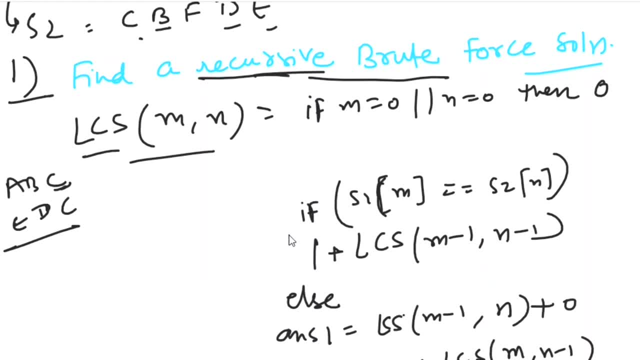 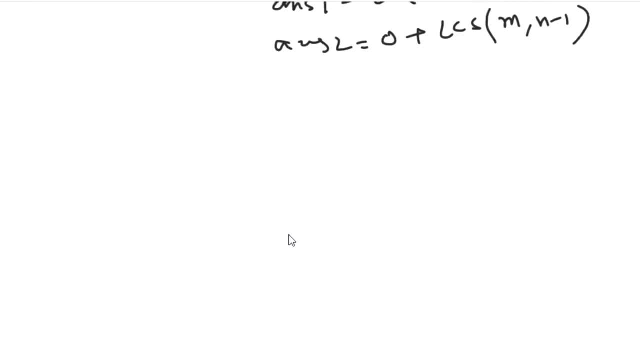 so this is our recursive solution. so we have found our recursive solution. but, as i've told you, you have to check for overlapping of sub problems before moving forward. so let's consider to string abcd and efgh. so if you try to implement this algorithm for this, these strings, then lcs of four comma four is lcs of macs off. 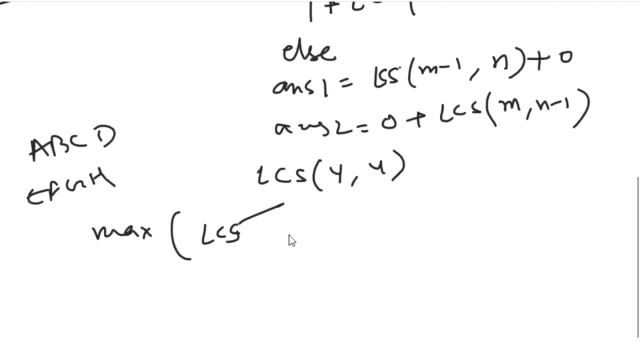 oh, okay, i forgot to tell you the question because of our 391 tell you that you have to take maximum of answer of let me draw a line so you have to return, since we have to return maximum length. so you have to take maximum of answer and answer 1 and answer 2. so lcs 4, comma 4 is maximum of. 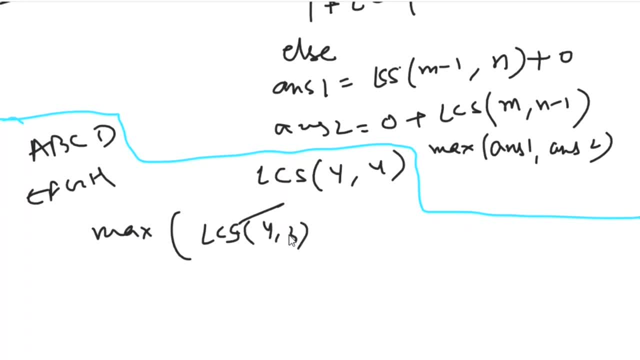 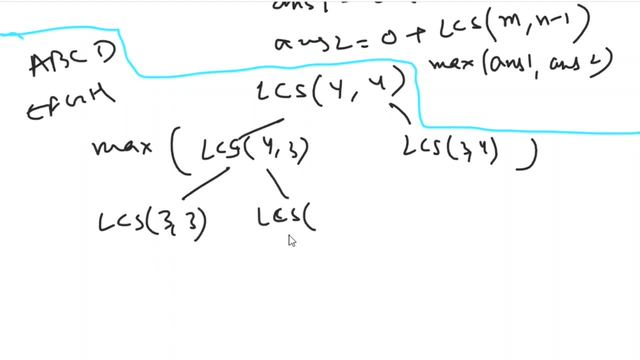 lcs 4 comma 3 and lcs 3 comma 4. okay. so now you solve it further. so it will be in lcs of 3 comma 3, lcs of what? 4 comma 2. okay, and it will be lcs of 3 comma 3. so you have to take maximum of them, remember. 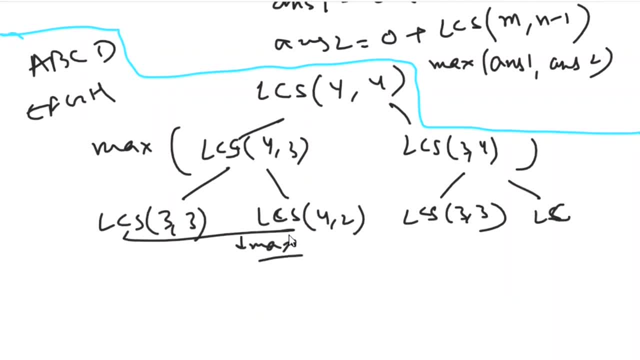 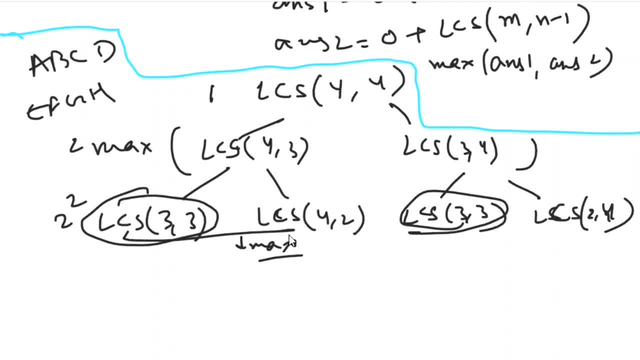 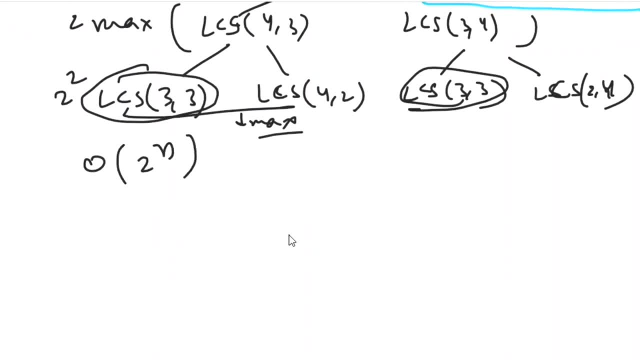 are increasing by a factor of 2.. So this is an exponential algorithm. Time complexity of this algorithm is O of 2 to the power n. So this will take us to our second step, that is, optimization of recursive solution. So let's see how we can do that. Okay, let me. 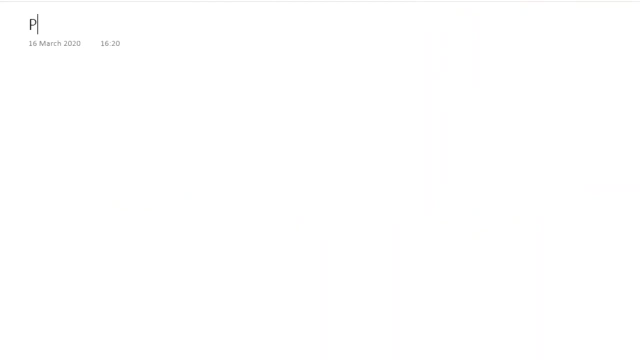 add a page, Page 4.. Okay So, as I have told you in the beginning of this video that you just first you have to check the number of arguments in your function. So LCS, m, comma, n have two arguments. Okay, So there can be m into n different subproblems. So you will need an. 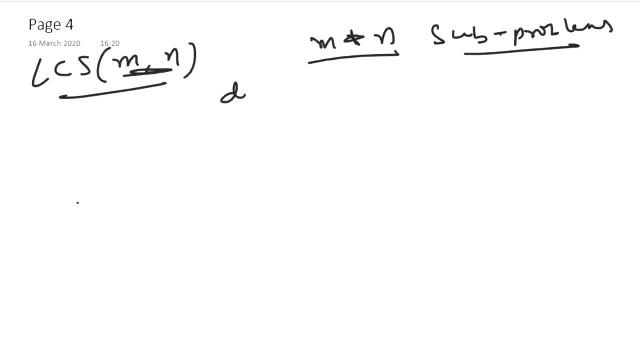 array of dimension 2.. So let's say you will need an array of dimension 2 and its size will be m and n. Okay, And you can initialize it to like minus 1.. So it will denote whether you have, if its value. 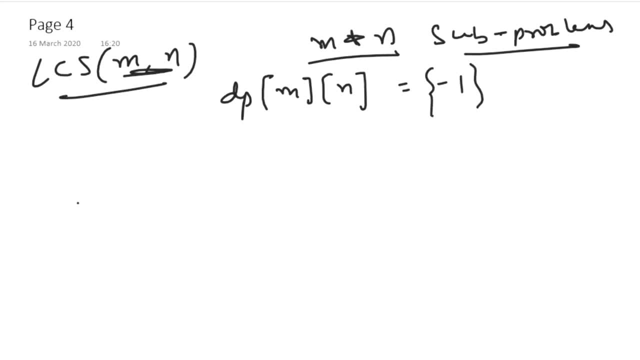 is not minus 1, then we have calculated the result of that subproblem. Okay, So now our LCS is this: So first we will write our base cases. as it is Base case, we will write Okay, Okay. So if it is not equal to minus 1, then we will simply return dp of m and n, because 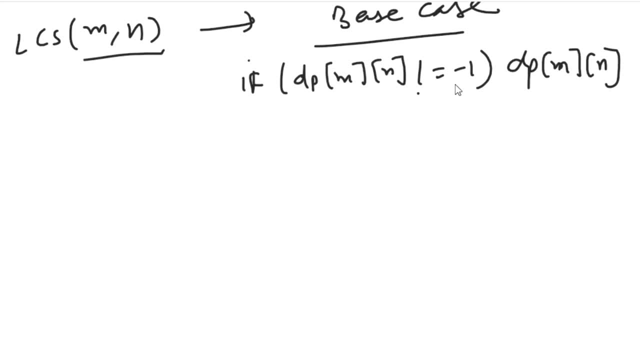 we have already computed it, And otherwise we will compute the results of both the cases, when s1 m equal to s2 n or it is not equal to, and we will finally get an answer and we will assign it to. Okay, So we will say dp m n and we will finally return dp m n, and okay, So this is our algorithm. 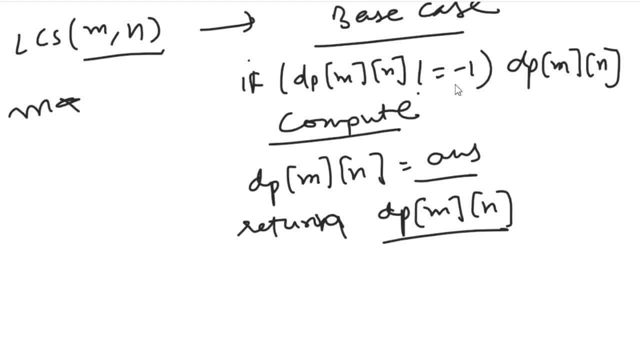 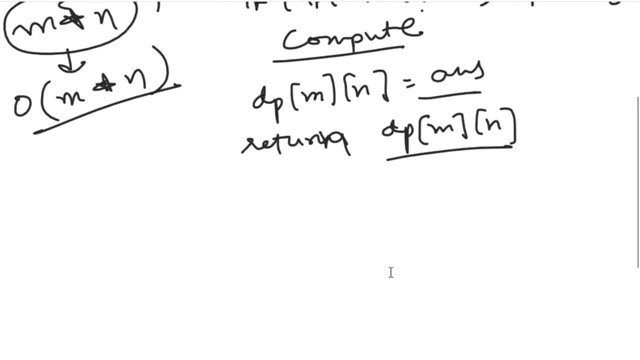 Okay, This is our final optimized algorithm. So, as you can see that we are solving only m into n distinct subproblems, and these are the maximum number of subproblems that are possible. Okay, and time complexity is O. Okay, so we have finished writing our algorithm. 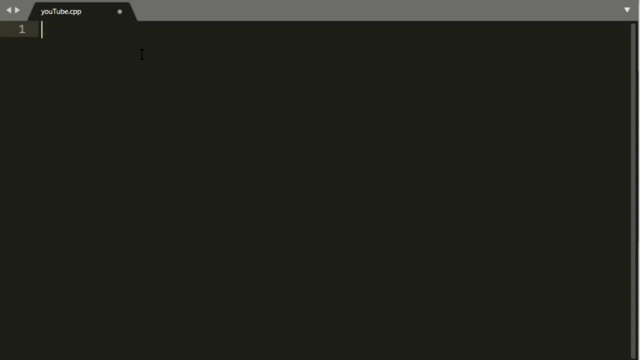 so let's write a code for it. So let's start with bids, standard C++h, and now using name std, and now we'll define our maximum length, And there will be two strings: Max, and then in dp: max, max, max. and now, man, come on. 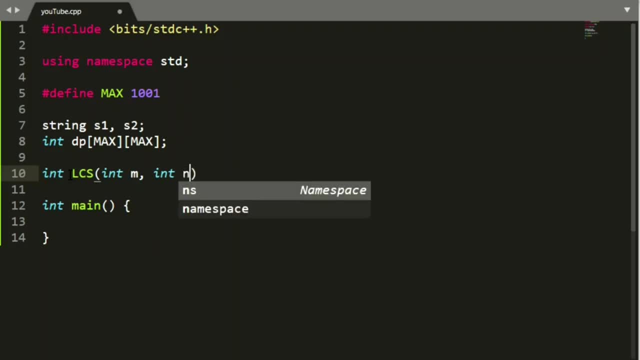 Int lcs, int n, int n. Now, if one of the m or n is 0, then we'll return 0.. This is our base case And otherwise, if Here is our output, which we have calculated, dp i j is not equal to minus 1, which means 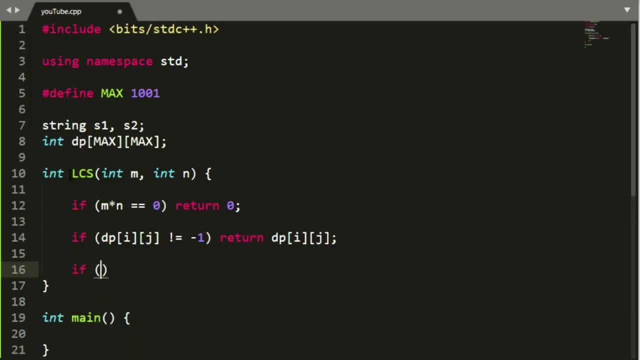 we have already computed the value. Then we will return dp i, j, And after that we have our condition for equal last characters. okay, In that case we'll return And assign simultaneously. So right now it will be M minus 1 because of 0 base. next thing, so DPM n equal to 1 plus max. 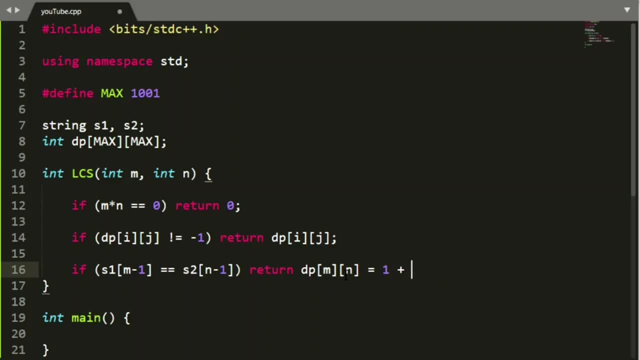 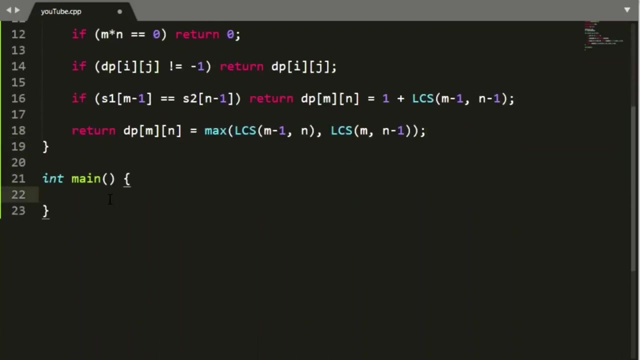 of norm max, it will be M minus 1 comma n minus 1, and our final case is will again assign and return simultaneously max of LCS M minus 1 comma n comma. LCS M comma n minus 1, and now we'll initialize DP array. okay, this is. 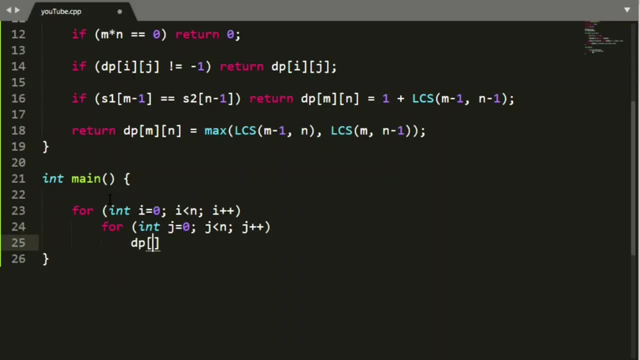 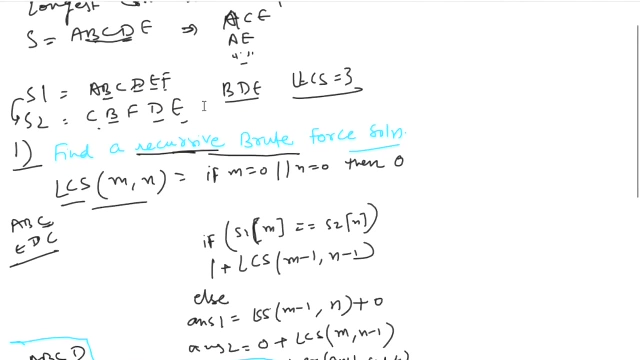 DP. I can use meme set for that, but I'll run this code in ID 1- and sometimes I even doesn't support me instead of them. so s1 is a, B, C, D, F and s2 is- let me check our example- C, B, F, D, E. so 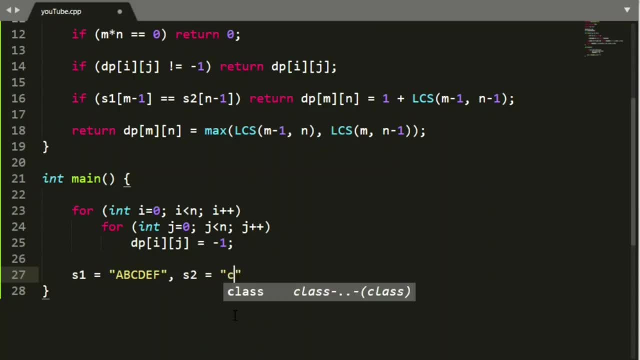 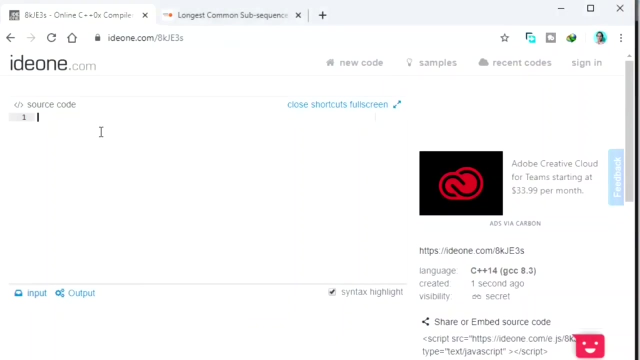 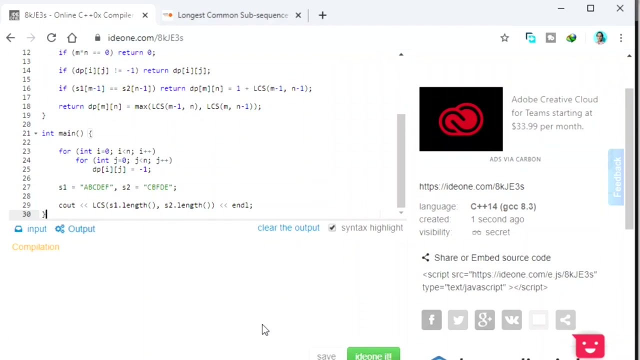 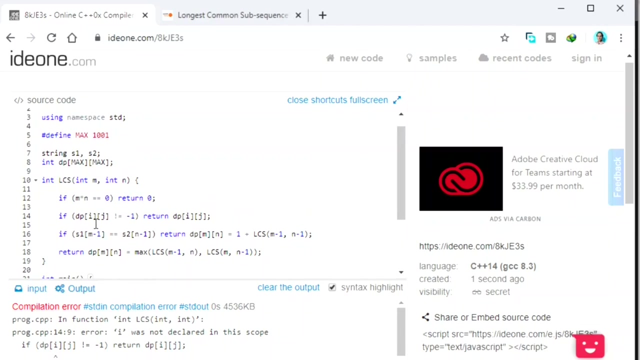 s2 is C, B, F, D, E and finally, we'll call our function LCS for s1 dot length and s2 dot length and we'll copy it. paste it in ID 1. so paste it now, ID 1 it. so there's some error. so yeah, ING are not defined actually. 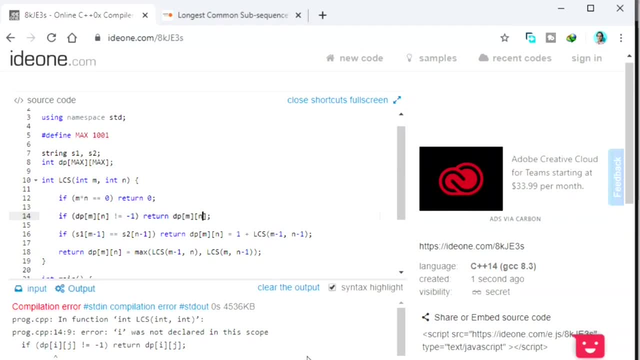 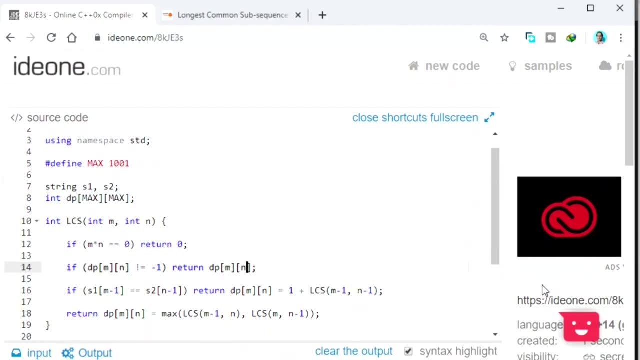 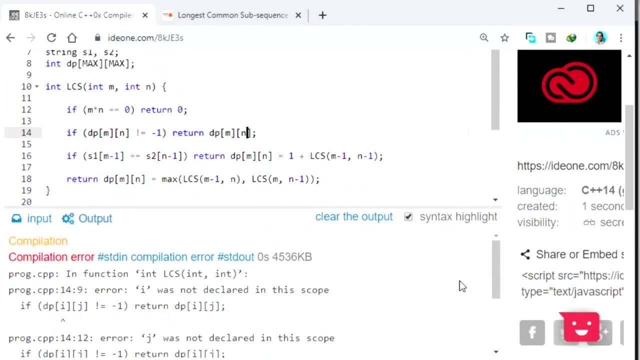 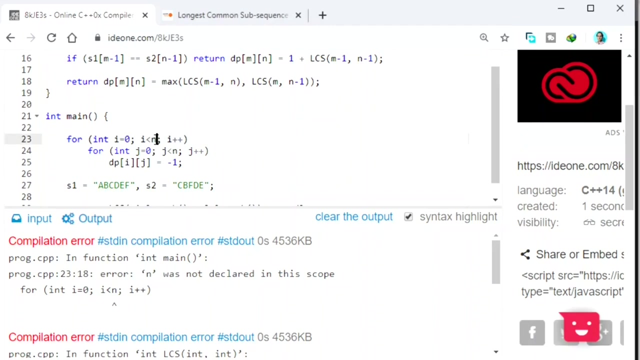 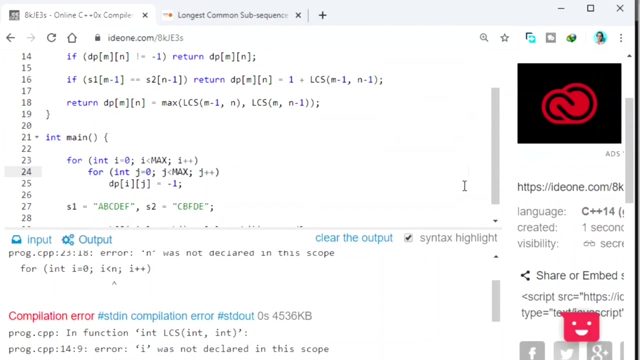 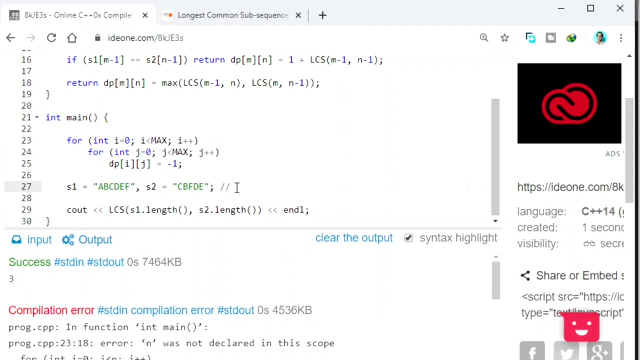 so M and and okay, so now ID 1, it again a compilation. it wait, wait, wait, no. yeah, there is no n, it was max, so I think it will work fine now. so, as you can see, we've got three years the answer. this is correct answer because we have B, D, E as the longest common. 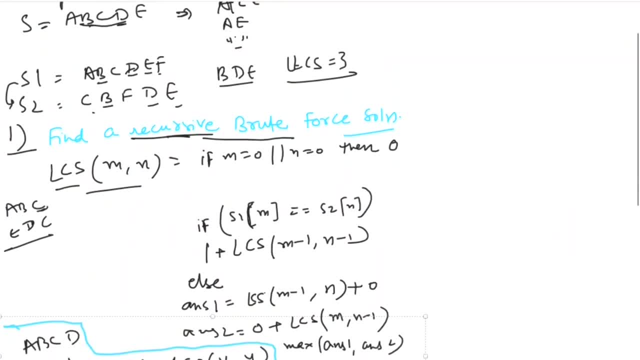 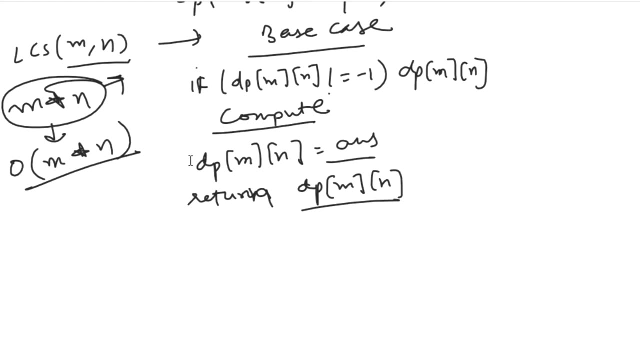 subsequence. so this is the code for it. yeah, this is code for it and this is our algorithm. so that's it, guys, for today. I hope you would have enjoyed this video and if you liked it, then please subscribe to my channel and like this video, share it with your friends. 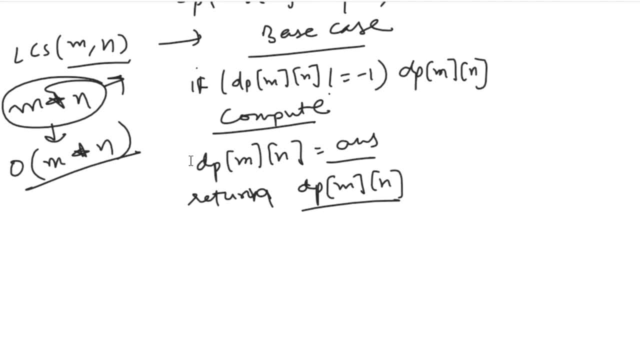 and also check out my blog. I'll mention the link in description. thank you guys. 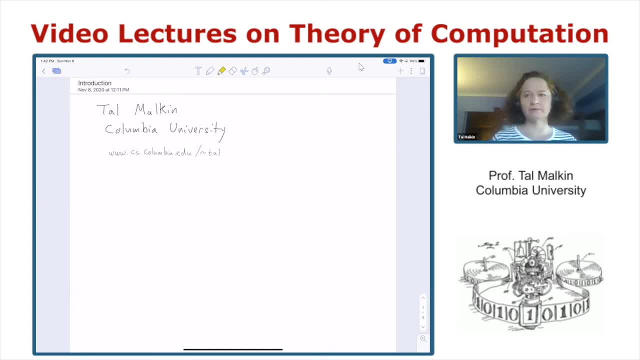 Hi everyone, I'm Tal Malkin. Welcome to this part of the lectures on theory of computation. I'm a professor at Columbia University in the theory group as well as in the security group. I got interested in computer science in general and specifically in theory of computer science. 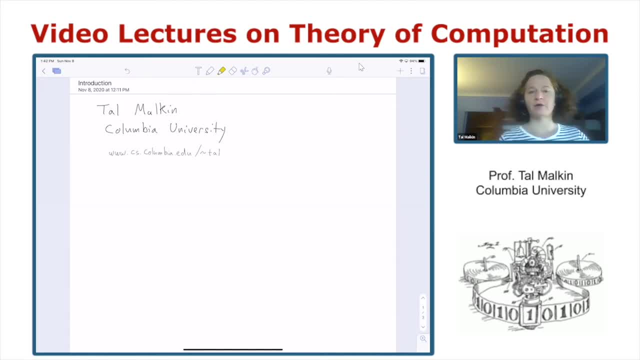 starting from math. I did my undergrad in Israel at Bar-Ilan University, where I majored in math and computer science, but math was really the thing I was passionate about. and then I took a class on theory of computation, similar to this class you're taking now, and I really fell in love with computer. 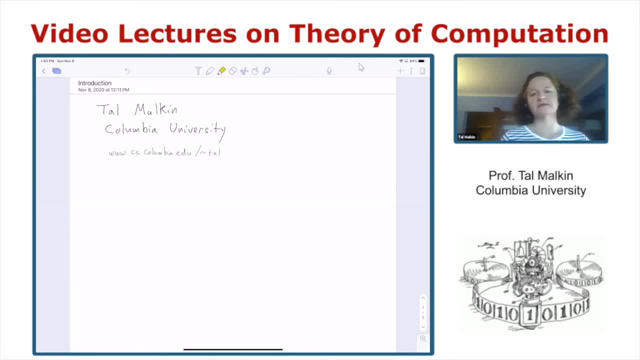 science. I then did my master's at the Weizmann Institute of Science in Israel on temporal logic, and then I did my PhD at MIT on cryptography, which is my main area of research. I then worked a couple of years at AT&T, at RL Labs Research. I've been at Columbia for over 15 years since then. 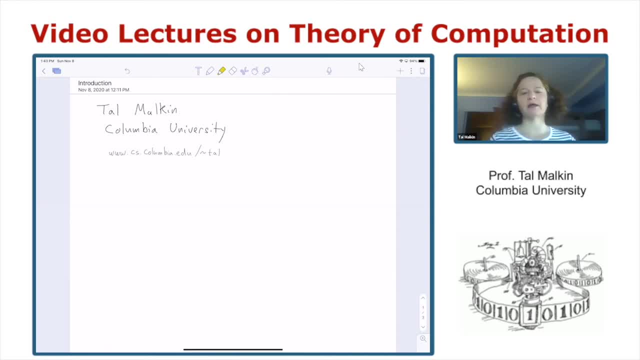 So just to say a word about my area of cryptography. it's an area within theory of computation and it's basically the mathematical foundations behind any applications requiring security or privacy. It's strongly related to complexity theory. in general, both cryptography and complexity theory have got a lot of feedback from each other. 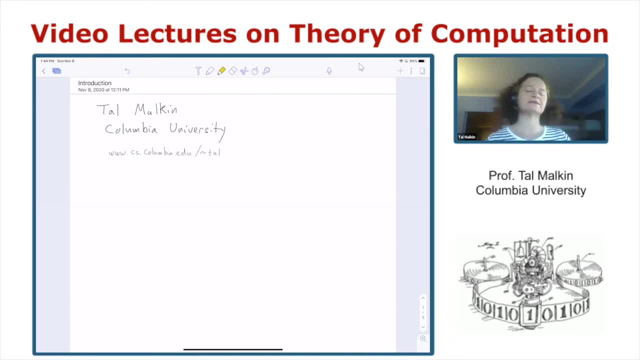 Just to give a very simple example: currently, what you're studying in the class is the limits of computation and what can and cannot be computed. The next part of the class you'll learn about complexity theory, which is basically what can or cannot be computed.